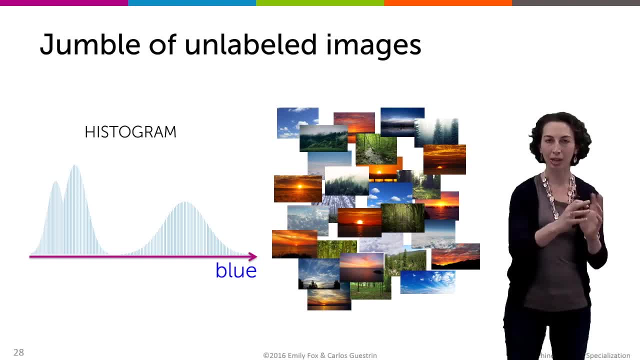 labels of our images. We can't separate and analyze each one of those classes separately to learn the parameters of those distributions. Instead, what we have is this pretty nasty space of intensities mixed over all these different images. So again, if we just look at the slice, 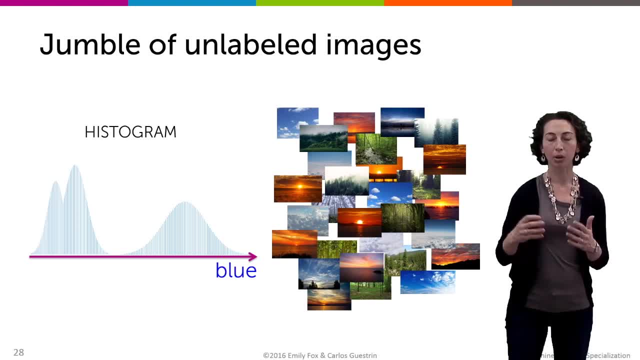 along the blue intensity value, then maybe our histogram would look like this three-hump distribution that we showed before. So this is just a histogram over values in our data set, but we're going to take a model-based approach and somehow we want to model this distribution. 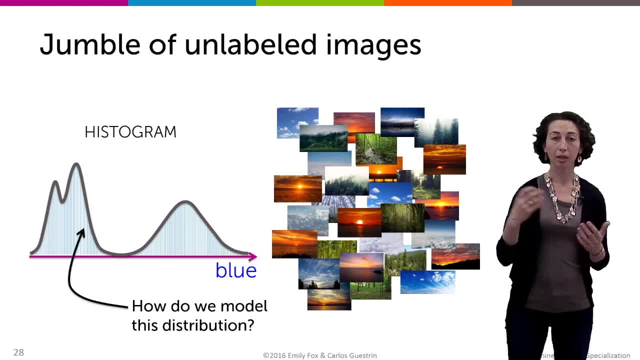 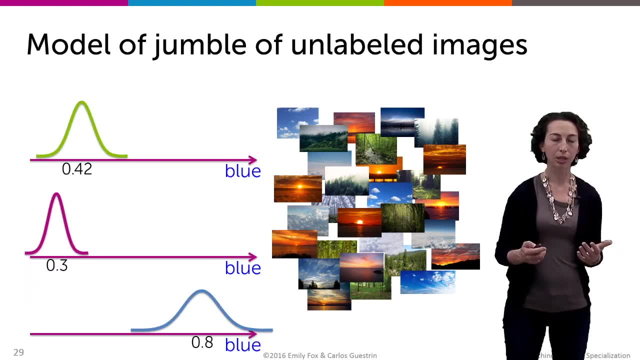 So the distribution over blue intensity in our entire data set. And a question is: how are we going to do this? Well, to do this, we're going to take each one of our category-specific distributions and simply average them together. So the resulting 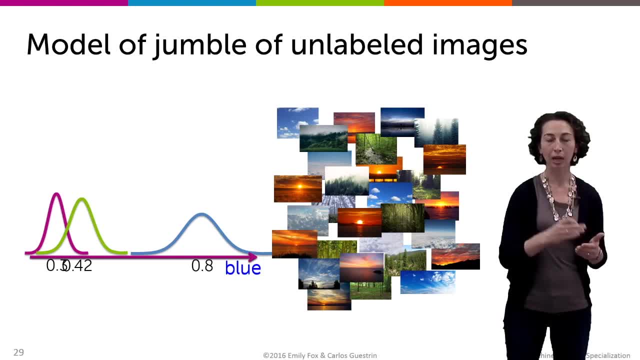 density is going to be an average of each one of these category-specific Gaussians. But this simple averaging assumes that each one of these different categories appears in equal proportion in our data set. So we have equal numbers of, let's say, two, three, four, five, six, seven, eight, nine, ten. 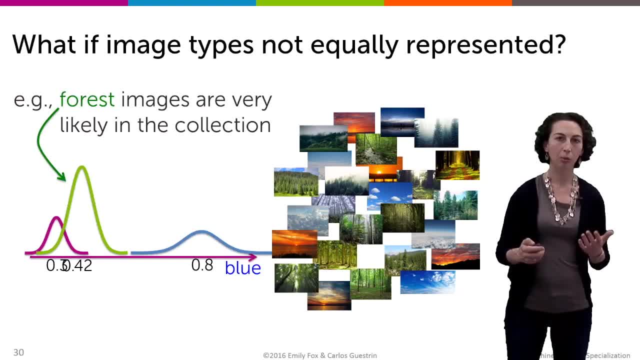 and ten. So we have equal numbers of sunset, cloud and forest images. But what if, for example, there are many more forest images than sunset or cloud images in our data set? Well, in that case we'd want to more heavily weight the forest distribution in this mixture, in this average. 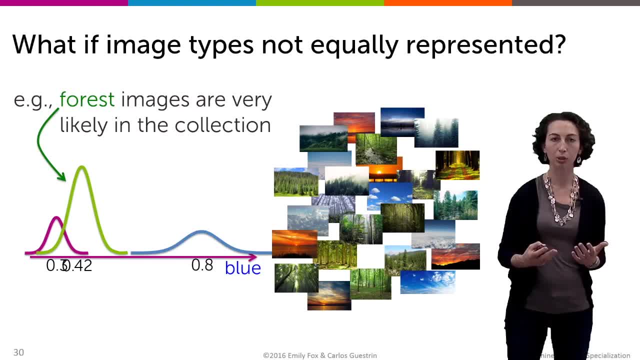 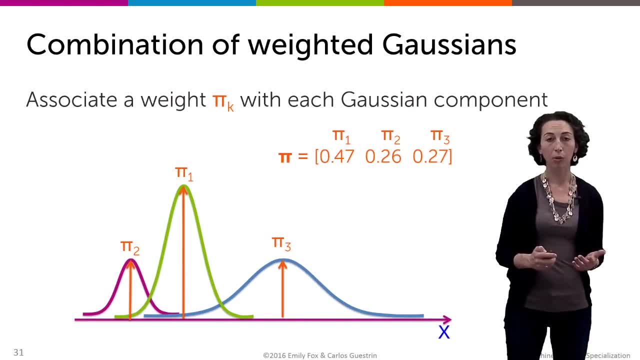 So we would do a weighted average over these different distributions, where the forest distribution gets higher weight in that average. More formally, we introduce a set of cluster weights, pi k, one for each cluster k. So in this example, where we're going to assume a, 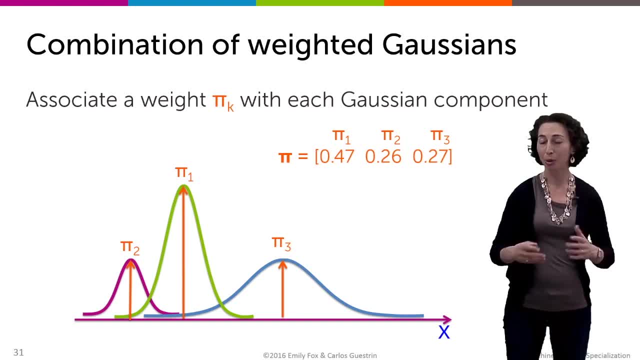 model with three different clusters, which happens to correspond to the truth, where we have forest clouds and sunsets. we'd have pi 1,, pi 2, and pi 3, where these weights are capturing the relative proportion of these images in our entire data set, And each one of these weights has to live between 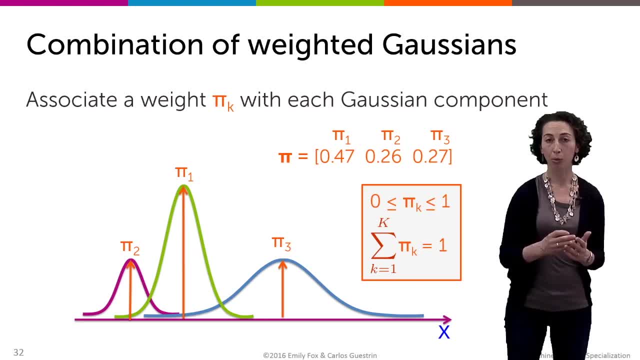 zero and one. So we're going to have a set of cluster weights- pi k- one for each cluster, k and one, And the sum of the weights across each of the clusters has to equal exactly one, And so what this means is when we're doing our weighted average- and these are the weights that 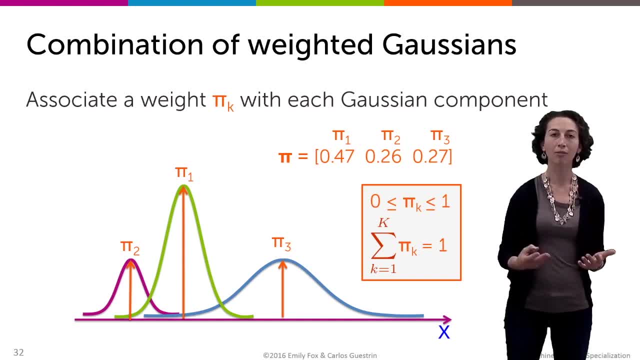 we're using in that weighted average. this is something that's called a convex combination. So remember- or I didn't actually mention this so you might not know it- but it's a distribution- a Gaussian is a distribution. So that means if we look at all the mass, if we increase or decrease the mass, the number of clusters, we're going to have about 1, and if we increase or decrease the mass, the number of clusters, we're going to have about 1.. or if we increase or decrease the mass, the number of clusters, we're going to have about 1.. 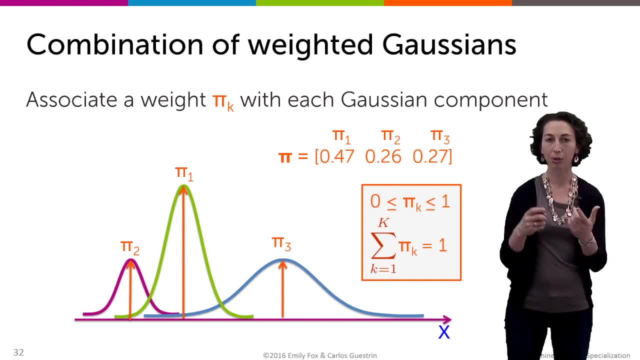 integrate over that distribution, over our random variable. the sum is one, probabilities add to one or in the continuous space, they integrate to one. Now, when we're looking at this mixture model, if because we're doing a convex combination of these individual Gaussians, 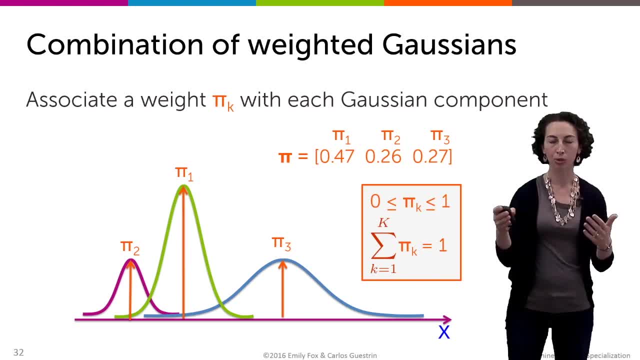 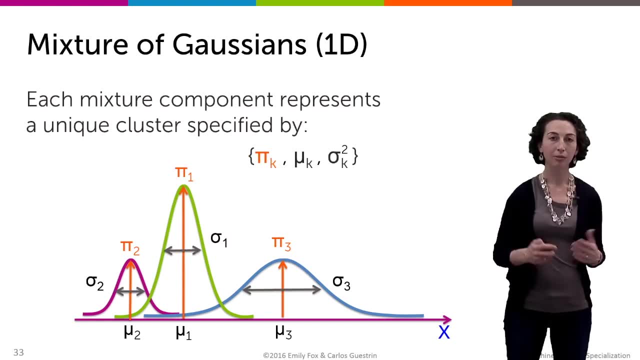 each of which integrates to one, then the overall result is still gonna integrate to one, so it still provides a valid distribution. And then, finally, to complete our mixture model specification, or mixtures of Gaussians in particular, not only do we have a mixture weight, 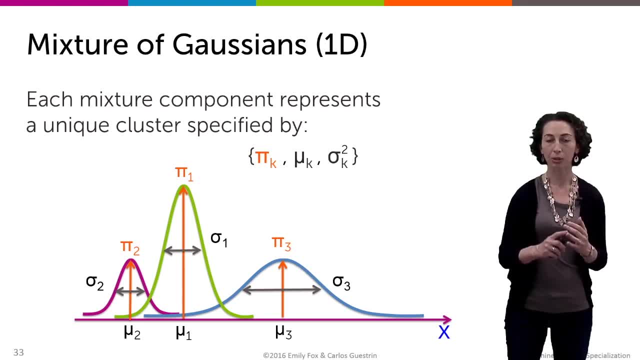 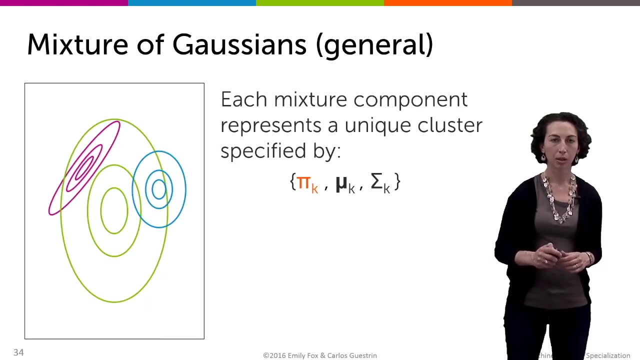 for each one of our different clusters. we also have a cluster specific mean and variance term in one dimension, And remember that those means and variances specify the location and the spread of each one of these different distributions that comprise our mixture model And when we're thinking about mixtures of Gaussians. 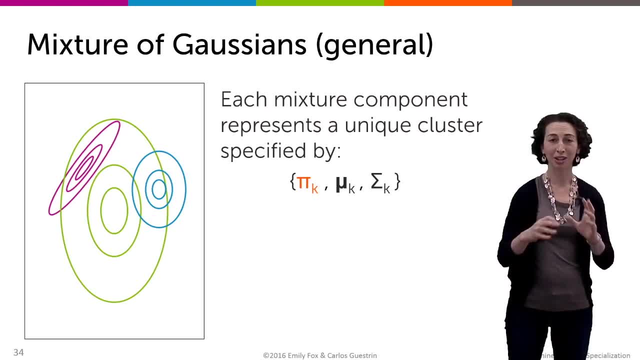 in higher dimensions. so I'm only gonna go up to a picture in two dimensions, not really the three dimensional Gaussians that we would be working with for this RGB vector, but two dimensions is as much as I can manage to plot. we end up with just a generalization. 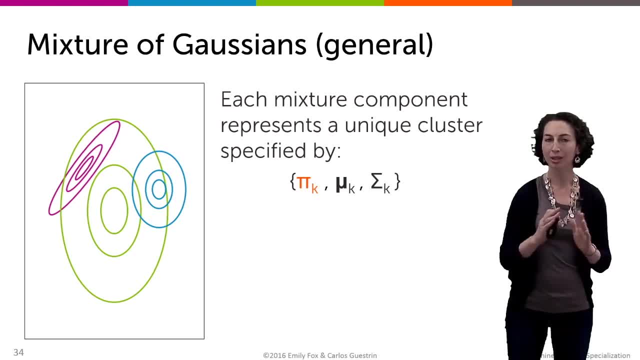 of the cluster parameters I talked about on the previous slide. The mixture weights are exactly the same. that doesn't change or vary with dimensionality. but now, instead of just a mean and a scalar variance, we have a mean vector and covariance matrix for each one of these Gaussians. 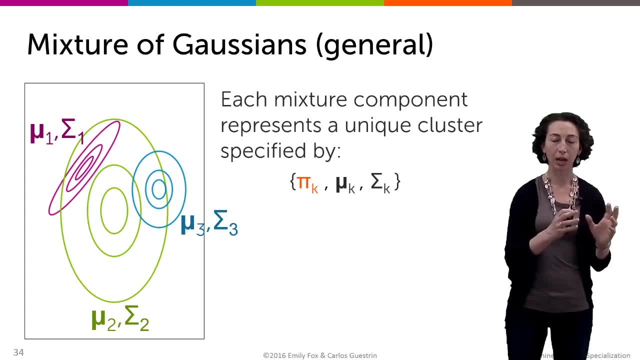 So remember, these means and covariances specify not only the location but also the shape and the orientation of these different ellipses. And then, when we're thinking about the mixture weights, it's pretty hard to annotate on these types of contour plots. 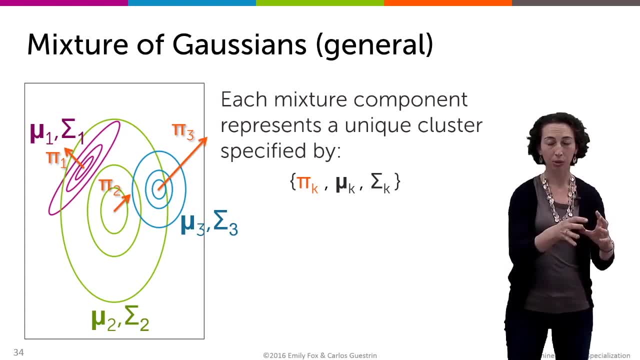 Just think of taking each one of these distributions, which are shown in these green, fuchsia and blue colors, and then weighting them, And this weight pi K is coming out of these. and then weighting them, And this weight pi K is coming out of these. 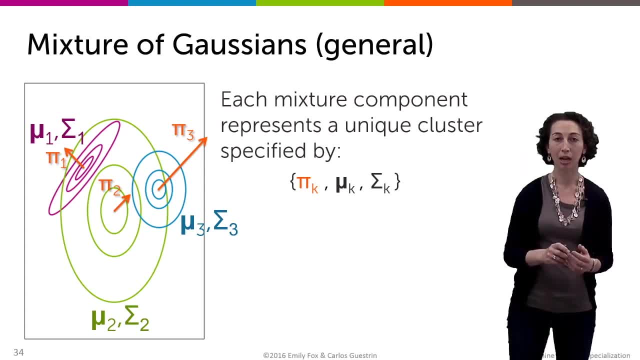 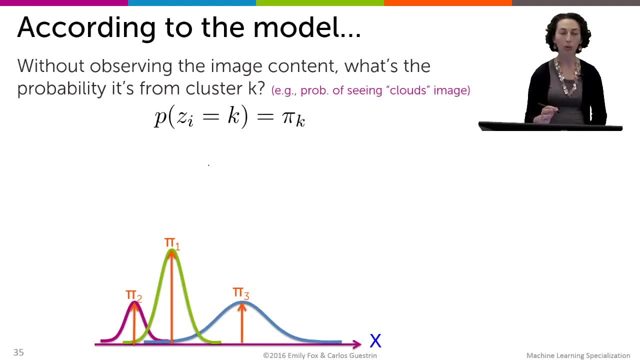 is coming out of the board, out of the slide here, And that represents how much we're emphasizing each one of these different mixture components in the overall mixture. And when we're thinking about using mixture models to do clustering, note that they can also be used. 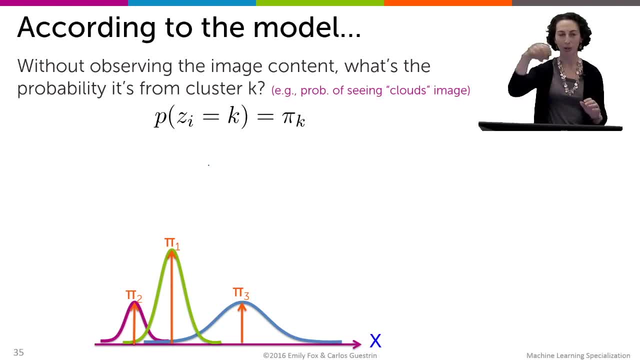 just to do what's called density estimation, so estimate those types of curves over the histograms that we drew earlier. But in our case we're gonna focus in on the clustering application, and there there's a really important other variable that we're gonna introduce. 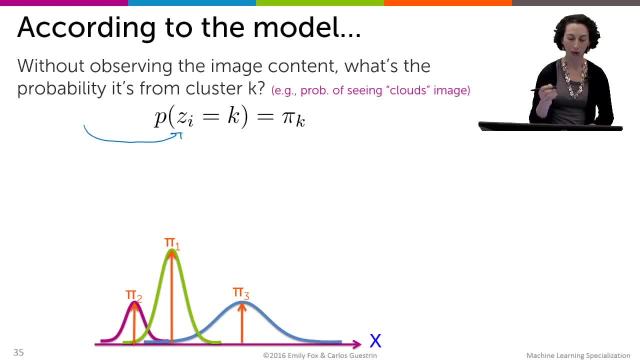 and that is the cluster indicator, the assignment variable for every one of our observations. So we have: this is the cluster assignment for observation xi. So this is exactly the same variable that we had in k-means, that was, assigning observations to clusters. 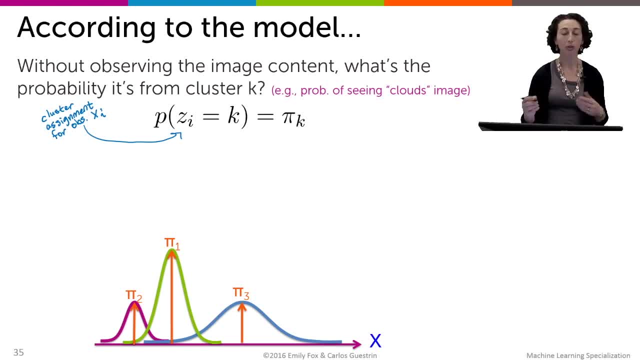 But in that case we're just using the cluster center. Okay, so let's step back and think about what our model is saying, And the first question we can think about is: what's the probability that the i-th data point in our data set is associated with the k-th cluster? 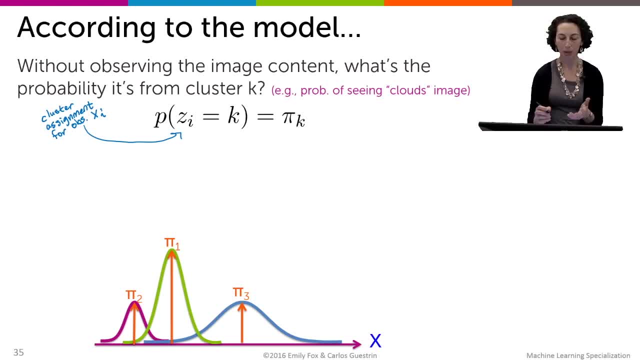 So, for example, when we're talking about our images, we could say: what's the probability that the i-th image I see is, let's say, in the cluster of Cloud's images, And let's talk about this before we've actually observed. 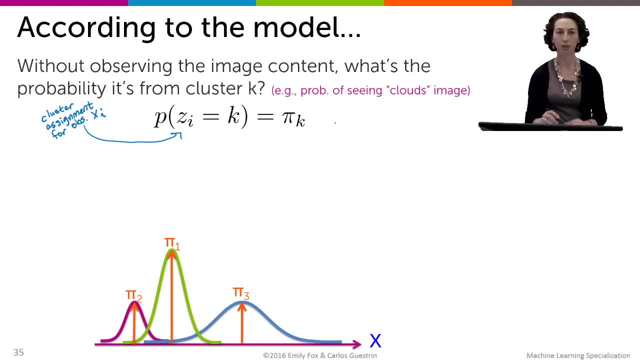 what the image is. All we know is it's the i-th index in our data set. Okay, well, this is fully specified by the mixture weight pi k, because that tells us how prevalent cloud images are in our data set. So that's given right here. 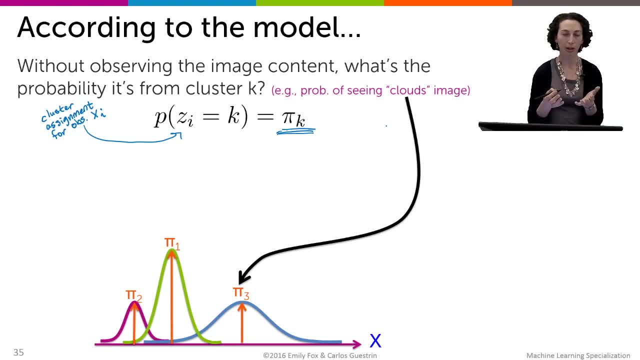 And if we don't observe the content of the image, then we just are caring about how many cloud images do we have relative to forest images, relative to sunset images? So we say that the prior probability that the i-th image is assigned to cluster k, 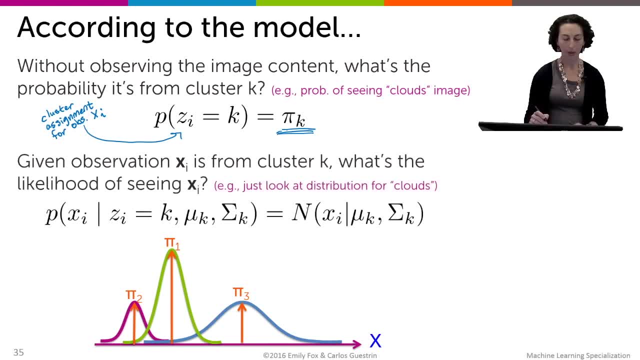 is given by pi k. Another question is: what if I know that an image comes from cluster k? Okay, so I'm gonna fix that. I already know that it's a Cloud's image. Now I can say what's the likelihood of observing. 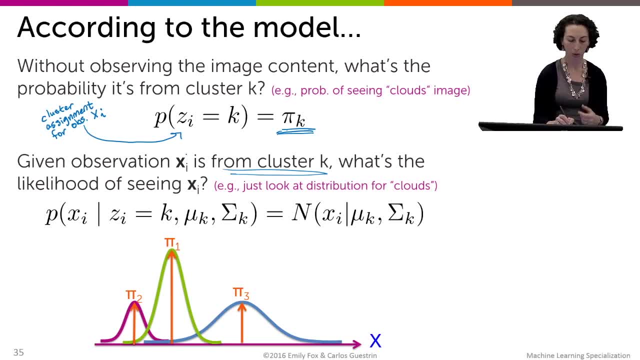 the RGB vector associated with this image? And what if I know that the i-th is assigned to X i, given that the image came from the k-th cluster, this cluster of Cloud images? And in this case, what we do is we simply go to. 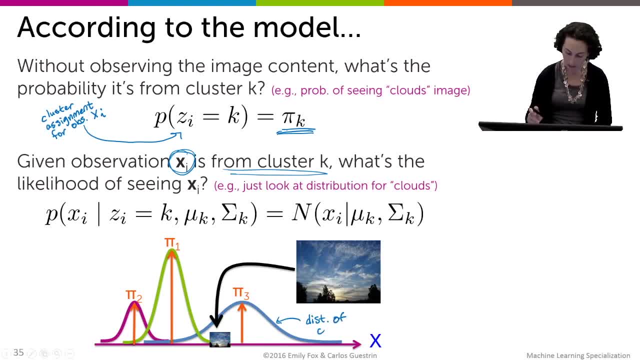 this is the distribution of Cloud images, or distribution of blue for Cloud images, And we say, okay, let's do this. let's take this one image I have- this is my Xi image- and I look at its blue intensity and I say, under this distribution for clouds, how likely is it? Well, it's pretty likely. 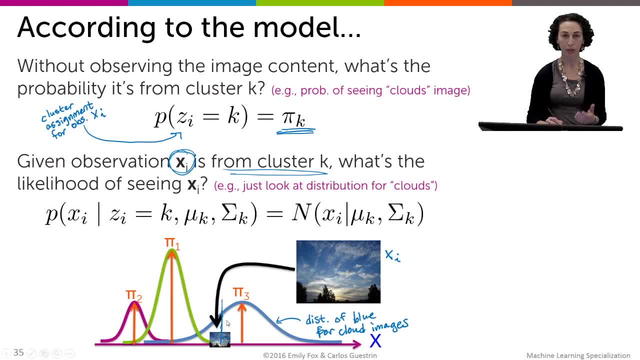 so it's a reasonable guess that, or it's reasonable to say that this was a cloud's image. but I can also look at this probability. under remember this was the forest category and I could say: well, what's the likelihood of this image under the forest category? Well, 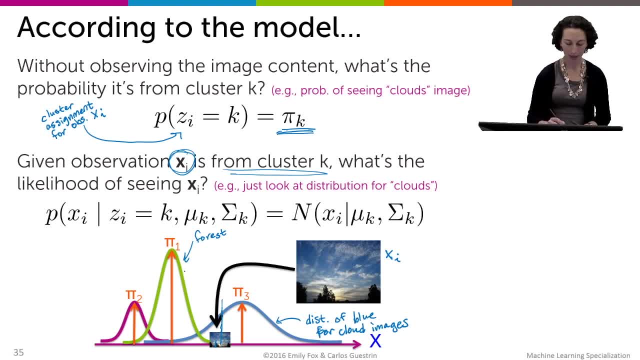 it's not that high, but, on the other hand, what we know is that there are many more forest images in our data set than cloud images. so what we're going to be doing when we're going to form our soft assignments- which we'll talk about in the next section- is we're going to be thinking about. 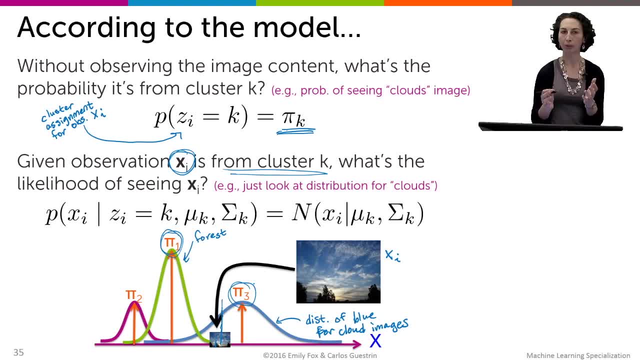 weighting these two terms, saying, well, what's the prior probability that this image is a cloud image or that this image is from any one of these different classes? So in this case it's most likely a forest image. but then I say, okay, well, now I've observed the content of this image, the